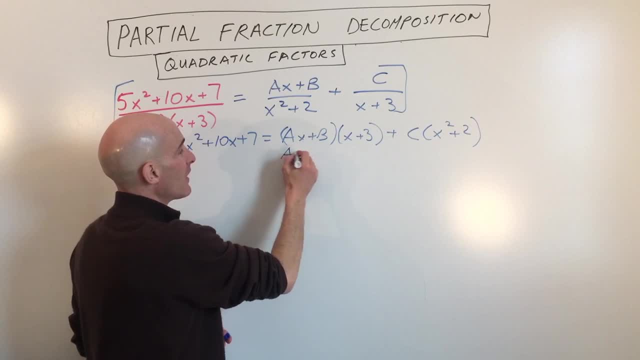 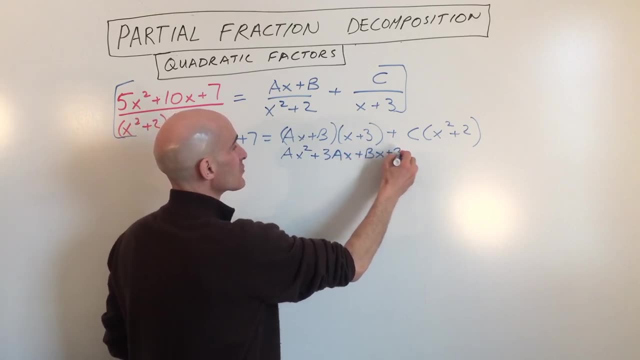 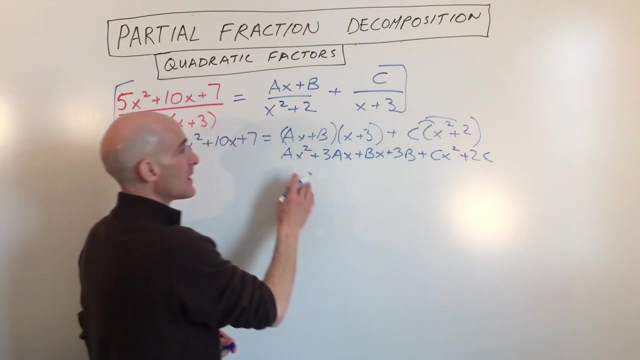 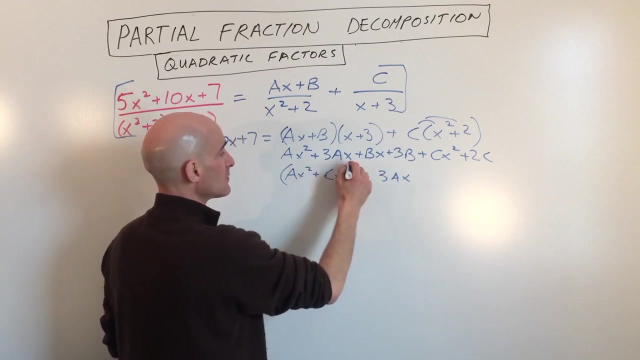 going to get a system. So first, let's foil this together, we're going to get ax squared plus 3ax plus bx plus 3b plus distribute the c here, we get cx squared plus 2c. Now what I want to do is I want to group together the x squared terms. So we have ax squared plus cx squared, I'm going to group the x terms together. So we have 3ax squared plus 3b plus 3b. Now what I want to do is I want to get 3ax. Okay, plus bx. Okay, and I'm going to group the constant terms together now, which 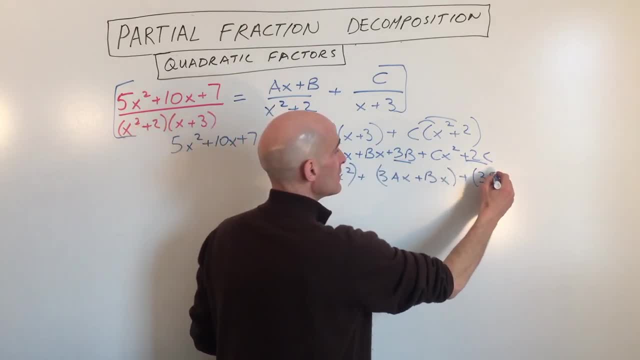 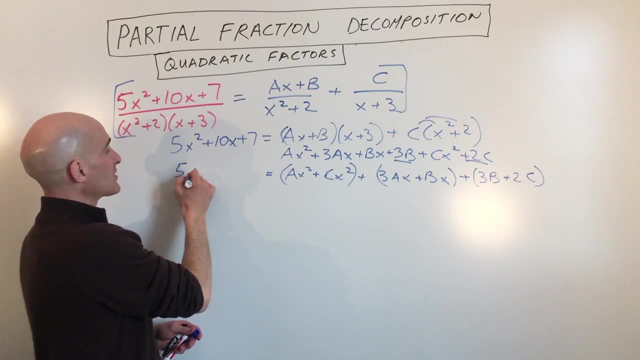 those are just going to be 3b and 2c. So that's 3b plus 2c. Okay, and that equals 5x squared plus 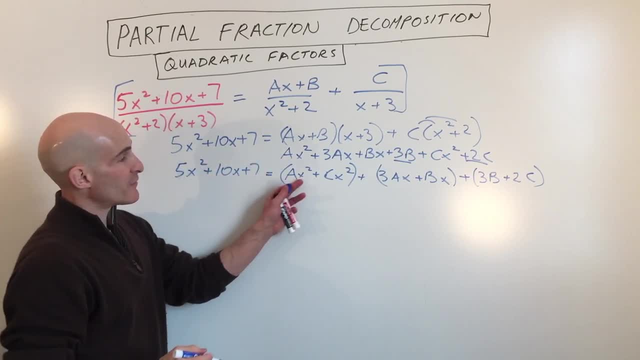 10x plus 7. Now what I'm going to do here is I'm going to factor out the x squared. So that's going 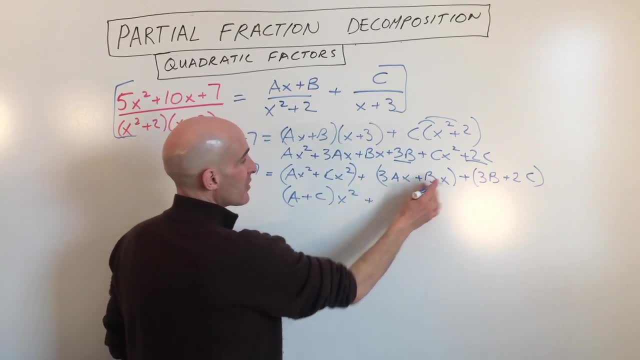 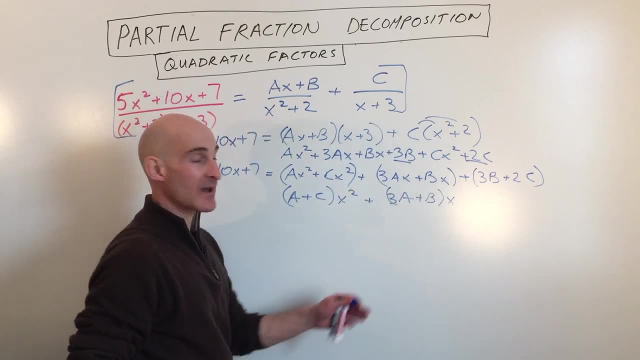 to leave us with 3a plus b times x. If you distribute the x back in, you get back the 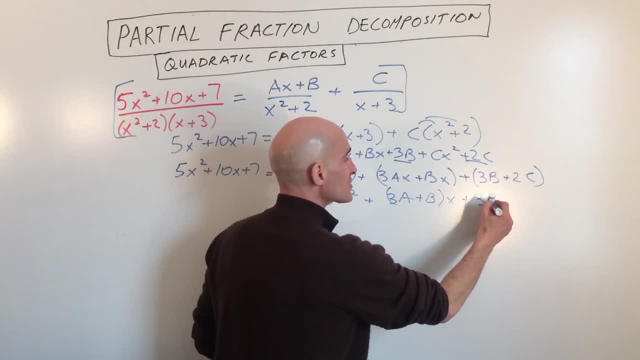 original here. And here, I'm just going to leave this as 3b plus 2c. Okay, now what we're going to 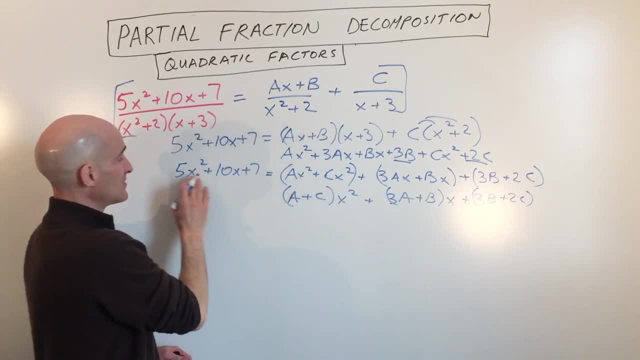 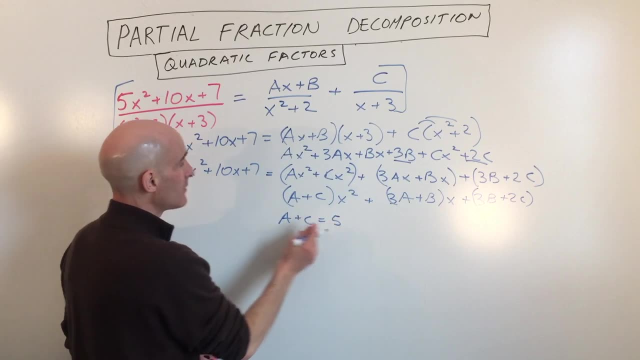 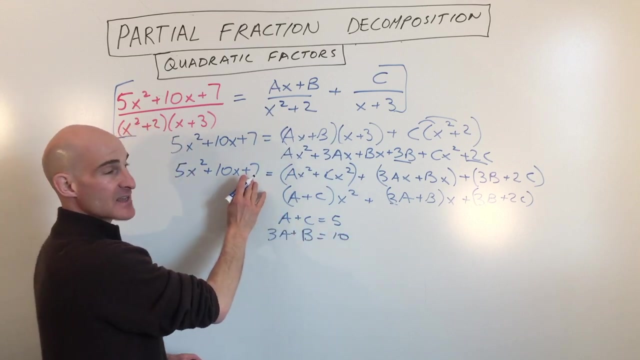 do is we're going to set, see, this is x squared, right? See, this is x squared, we're going to set a plus c equal to five. Okay, so a plus c equals five, we're going to set 10, see, 10x, here is x, we're going to set this coefficient equal to this coefficient. So we have 3a plus b equals 10. And then the constant seven, we're going to set equal to this constant on the right side, 3b plus 2c. So we have 3b plus 2c equals seven. So now you can see what we have 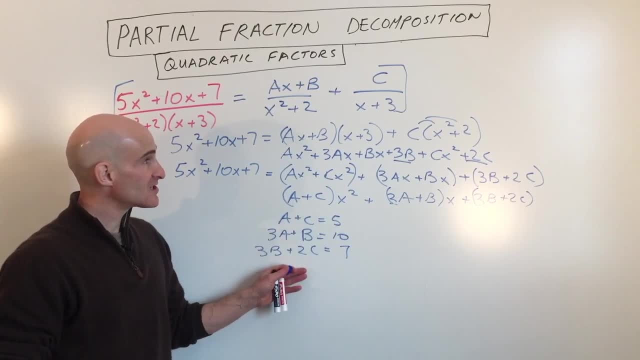 here is we have a system of equations, we're going to solve this system, and we're going to find our a, b, and c. 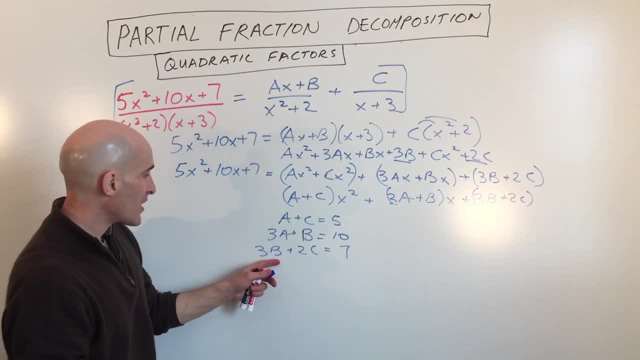 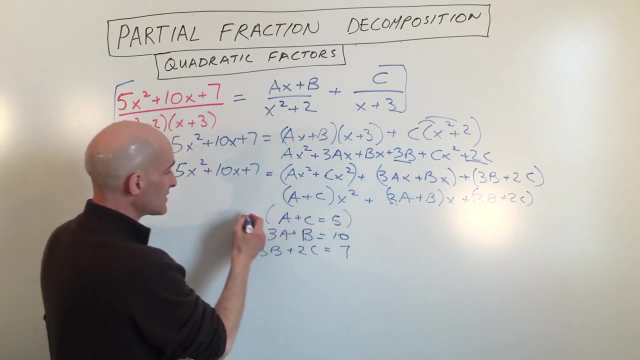 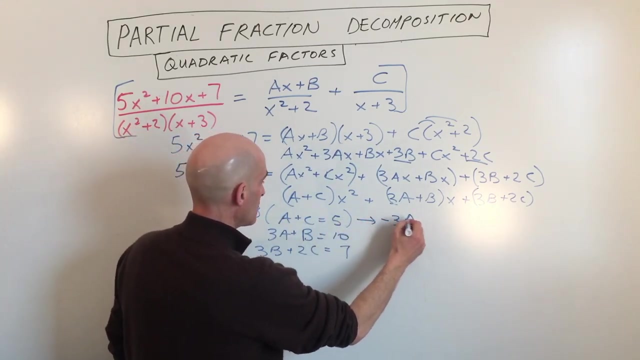 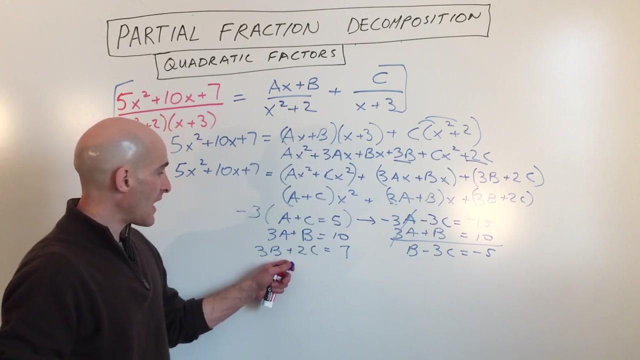 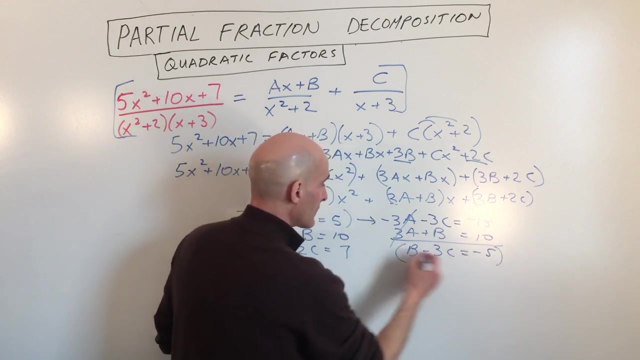 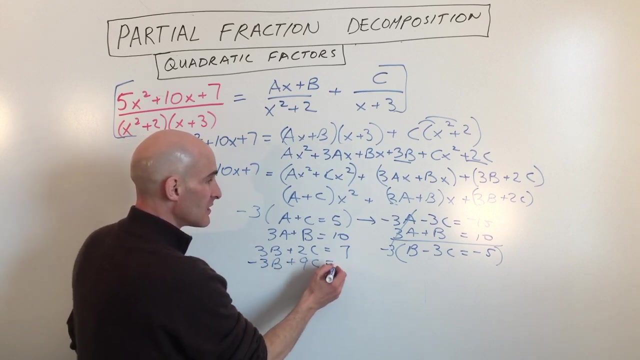 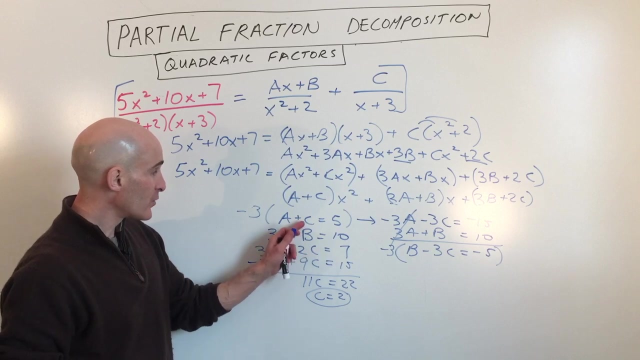 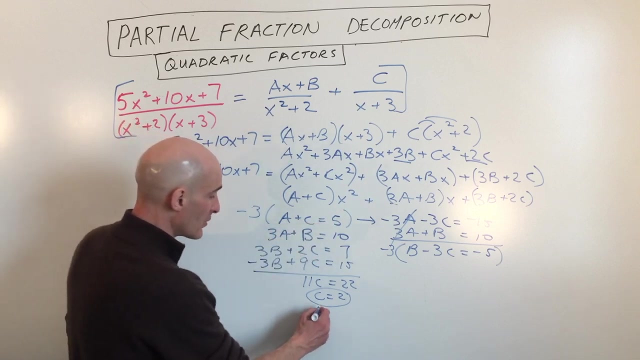 So let's take a look at this system. So what should we try to eliminate here? Well, let's see, we've got a, a, okay, we've got b and b, we've got c and c. Okay, so what should we do to eliminate this? Why don't we multiply this first equation times negative three? Okay, so if we do that, we get negative 3a minus 3c equals negative 15. I'm going to add it to this equation here, 3a plus b equals 10. If we add those together, you can see the a's are going to cancel, and we get b minus 3c equals negative five. Okay, so far so good. So now we're going to combine these two equations together, they just have b's and c's, okay, to solve for either b or c. So why don't we multiply this equation here times negative three and combine it with this equation. So if we do that, multiply by negative three, we're going to get negative 3b plus 9c equals 15. So if we combine these together, we get 11c equals 22. So now we know c equals two. If we take the two and we work our way back, let's put two in here, we get, well, we could put into any one of the equations, really, if we know c is two, let's put it into this equation. That means a must be three. Okay, so now we know a equals three. 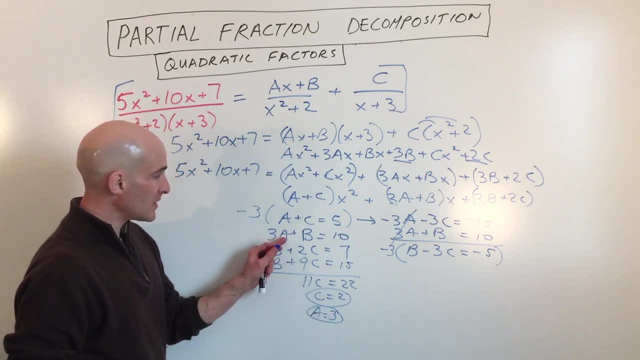 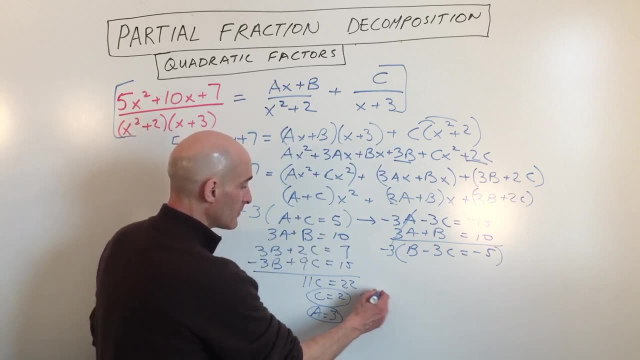 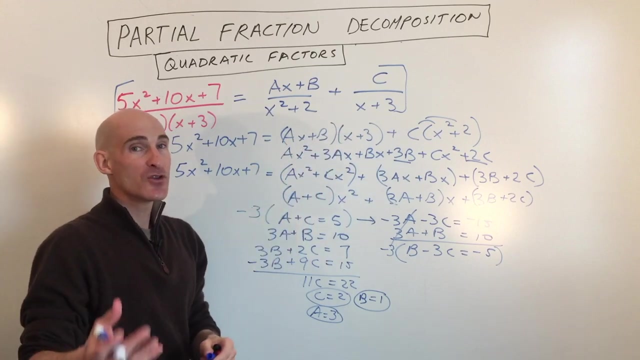 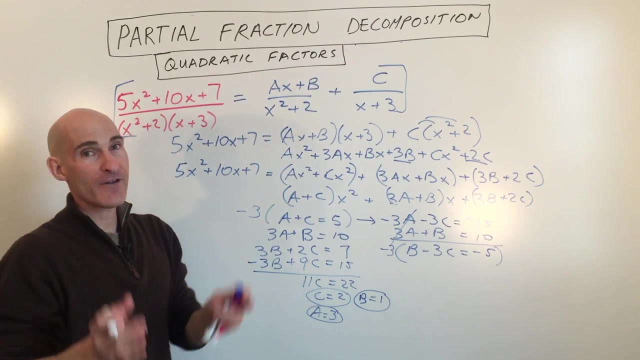 We just have to solve for b. Okay, if we know that a is three, that's going to be three times three is nine, which means that b must be one. Okay, so b equals one. And now we have our a, b, and c. We can put those back in for a, b, and c here, and these are going to be our partial fractions. You can check your work. If you get a common denominator and combine these into one fraction, you can verify that you get back this original fraction. So this has been how to do partial fraction decomposition when you have a quadratic, meaning a second degree factor. I'll see you in the next video.